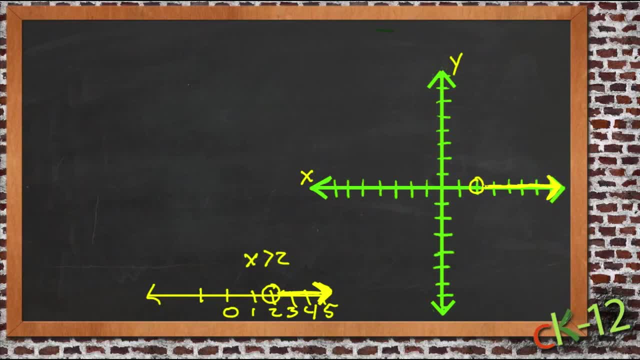 But all I'm showing here is that x is greater than 2 and y is zero. Since we aren't specifying what y can be on this graph here, we could also graph this same line right here and be just as accurate, because we're only talking about what x can be. We could graph it down. 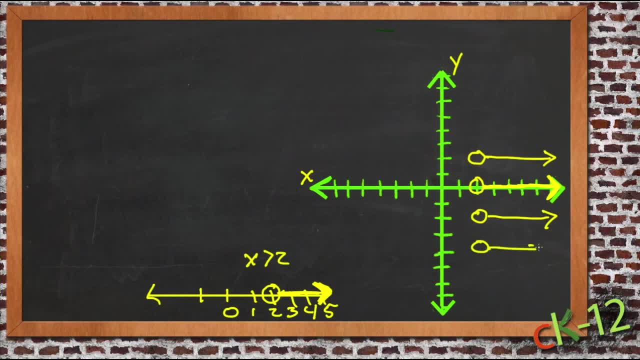 here and be just as accurate. In fact, we could graph it anywhere we wanted: vertically, all the way down there, as far down as we wanted to go, and all the way up as far as we wanted to go, as long as the x coordinate of whatever point we were graphing was the same as the. 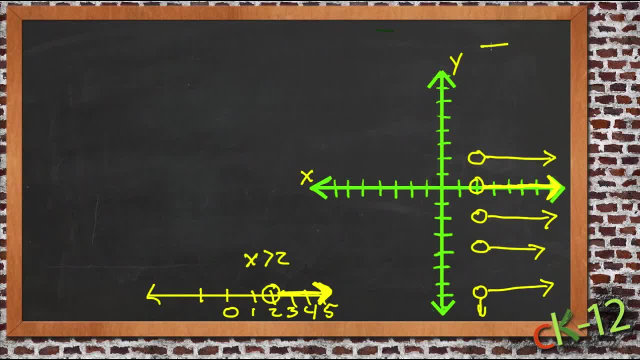 y coordinate, or even if the x coordinate of whatever point was greater than 2, it would be on the graph of that expression. So really, here, what we're doing is starting at 2, leaving an open circle. In this case, we use a dashed line to show that open circle. 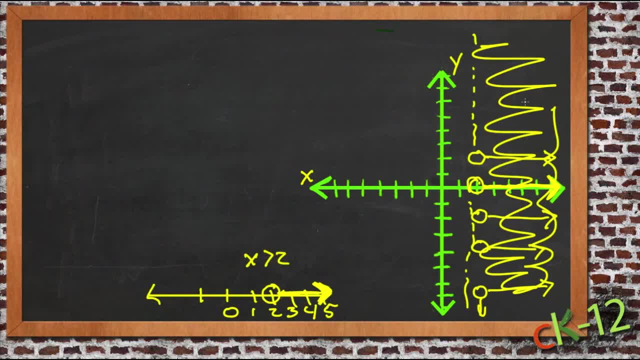 goes vertically, and then we shade everything to the right Because anything y wants to be, it can, as long as x is greater than 2.. So let's see how that applies to a question sent in by a student. Kisho here said that she needs to write the absolute value of x. 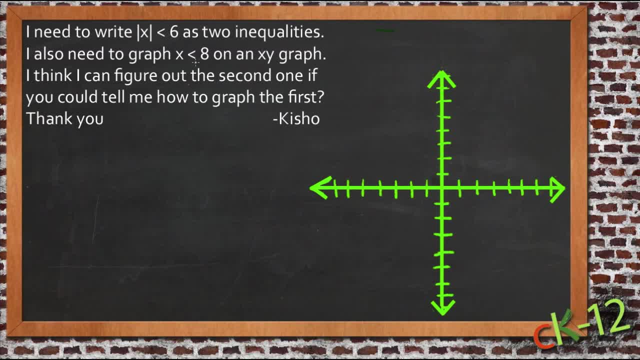 x is less than 6 has two inequalities, and then she needs to graph: x is less than a on an xy graph. She thinks she can figure out the second one if I can tell her to do the first. So first let's write the absolute value of x is less than 6, and then we'll graph it. 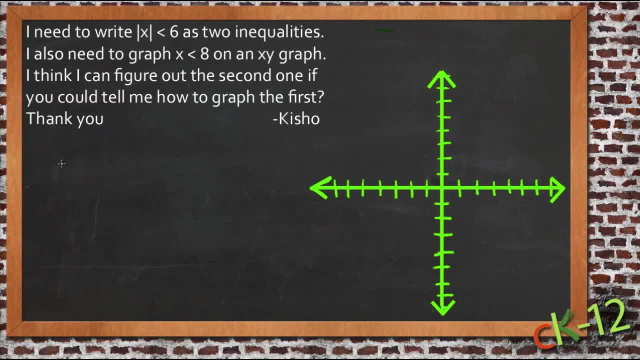 and we'll leave the other one for her to graph. So if I have the absolute value of x is less than 6, then what I'm saying is that, whether x is positive or negative, the value of that number can't be 6 or anything bigger. 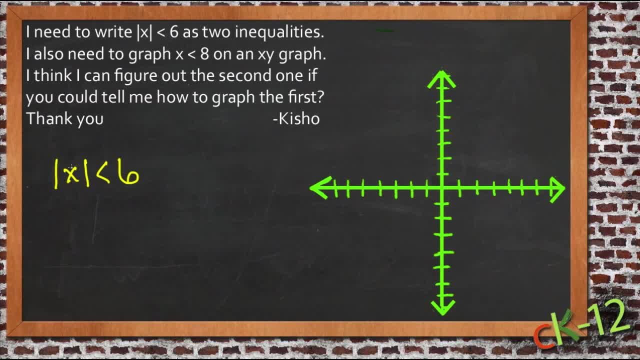 So in other words, x can't be less than negative 6, because then it would be a bigger number than 6 inside of here, and it can't be greater than regular positive 6, because then that number would be bigger than 6 in there. 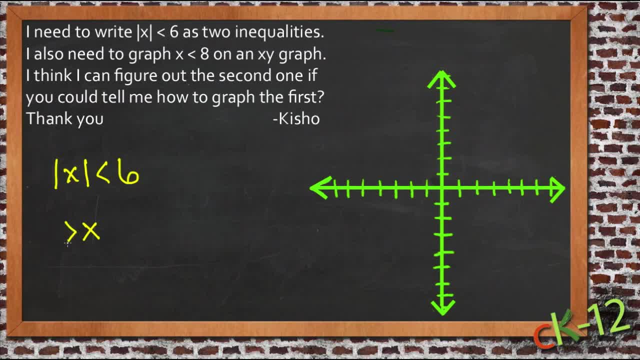 So we need to say: x is greater than negative 6, so less negative than negative 6, but also less than positive 6.. x is all the numbers in between negative 6 and positive 6.. Not more negative, Not more positive than this and not more positive than this.